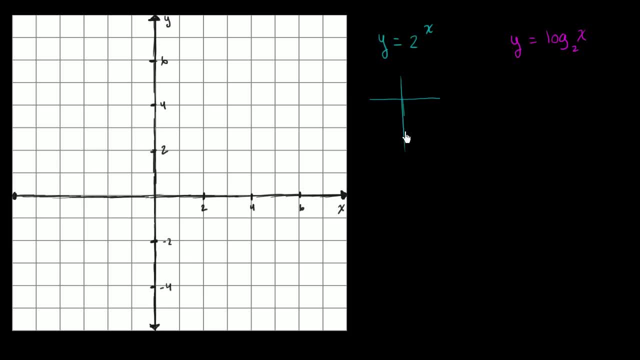 I'll make a little table here, different x values and the corresponding y values, x and y. we can start with negative 2, negative 1, 0, 1, 2, 3.. In each case y is going to be 2 raised to this power. 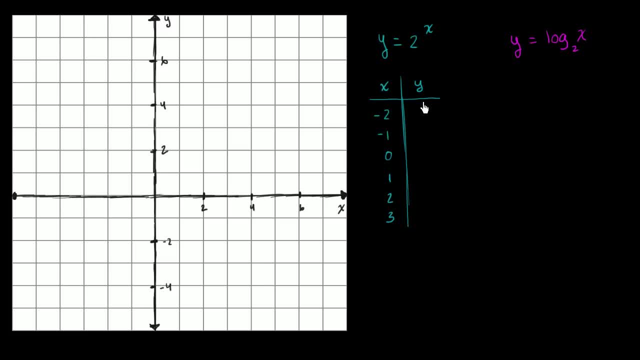 2 to the negative 2 power is going to be 1. fourth, 2 to the negative 1 power is going to be 1. third, 2 to the negative 2 power is 1. half. 2 to the 0 power is 1.. 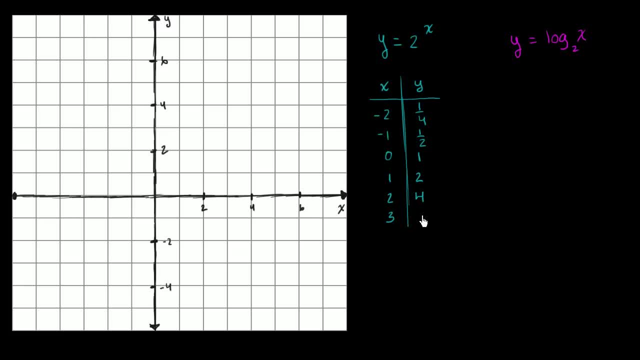 2 to the first power is 2.. 2 to the second power is 4.. 2 to the third power is 8.. Let's graph that: 2 to the third power is 8.. 2 to the third power is 8.. 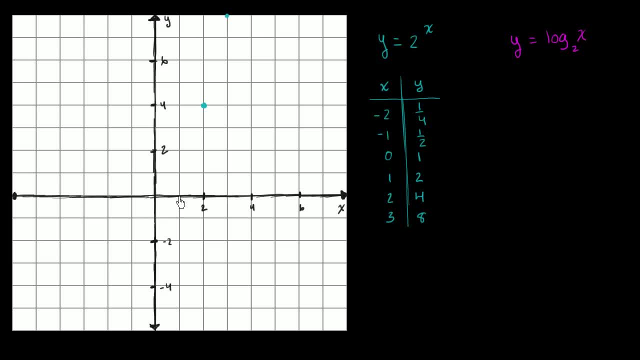 2 to the second, power is 4.. 2 to the first power is 2.. 0-th power is 1.. 2 to the negative: 1 power is 1. half. 2 to the negative: 2 power is 1. fourth, 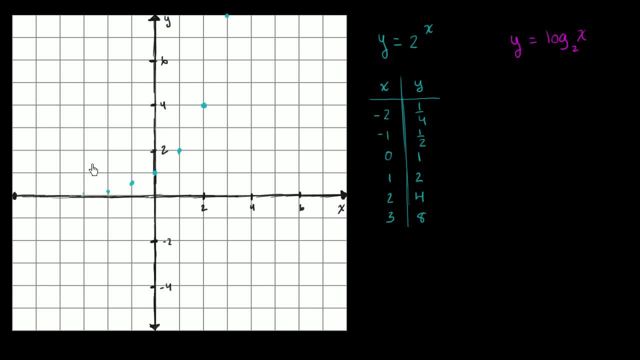 We'll get even a 2 to the negative. third, power is going to be 1- eighth. So it's going to look something like this. So the graph is going to look something like this right over here And it's kind of your classic sometimes, this: 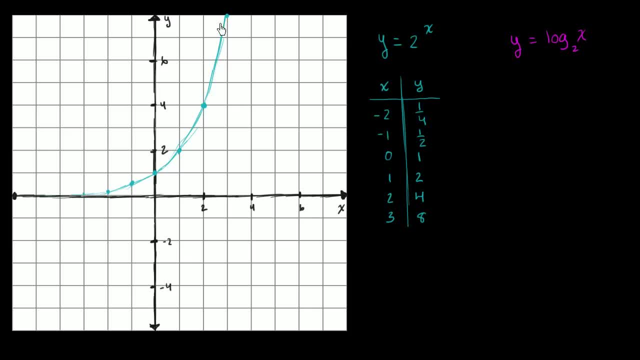 will be called your exponential hockey stick, because it kind of looks like a hockey stick, where it just kind of starts kind of slow and just bam, shoots straight up And notice, as we go to the left, as x becomes more and more and more negative. 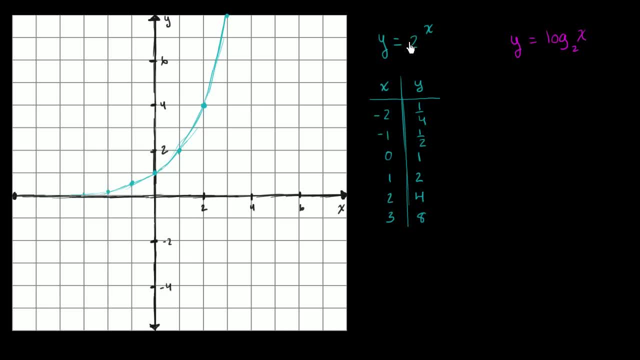 our value approaches 0, but never quite gets there. If we have 2 to the negative 1 millionth power, it's going to be a very, very small number, very, very close to 0. But it's not going to be quite 0.. 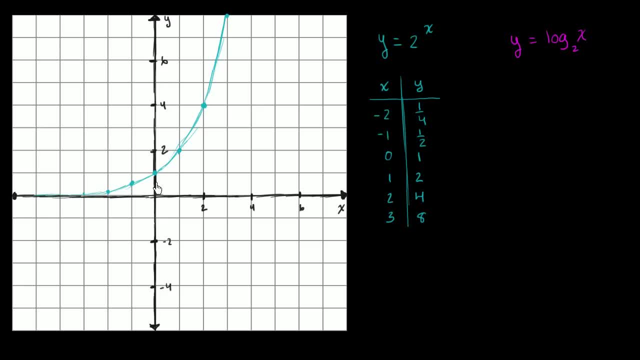 So we're going to have a horizontal asymptote at y is equal to 0, or the x-axis is a horizontal asymptote. Fair enough, Now let's graph: y is equal to log base 2 of x. And before I graph that, let's just 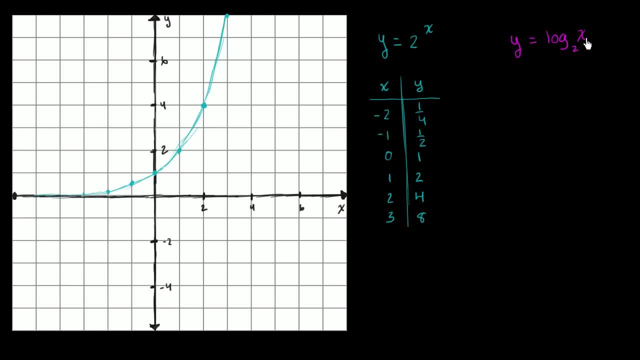 think about another way of representing it. This literally says: for any x, what power? what exponent y? if I raise 2 to that would give me x. So this is an equivalent statement, as saying 2 to the y, power is equal to x. 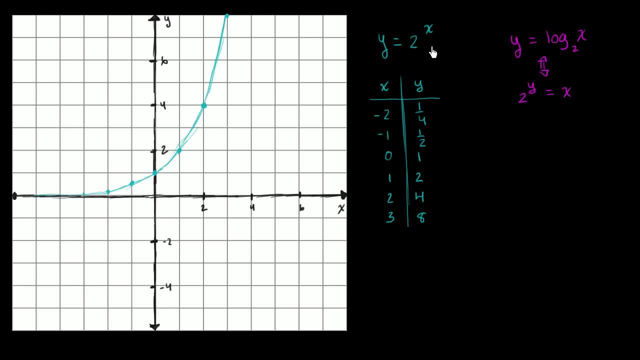 And if you notice what we've done here, between these two things, you're essentially just switching the x's and the y's. Here it's 2 to the x, power is equal to y. Here it's 2 to the y, power is equal to x. 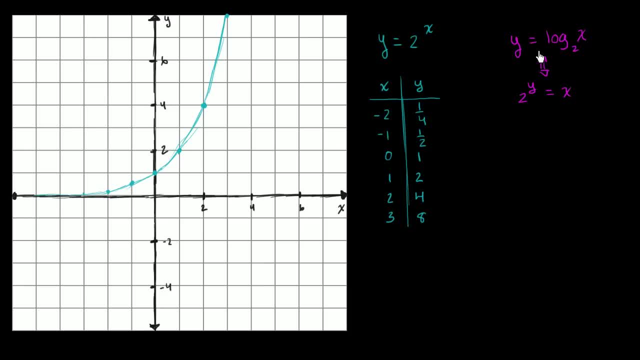 So, really, this and this, you've swapped the x's and the y's. So you've swapped the x's and the y's And what we will see is that we could essentially swap these two columns, So x and y. So let me just do 1, fourth, 1 half 1, 2, 4, and 8.. 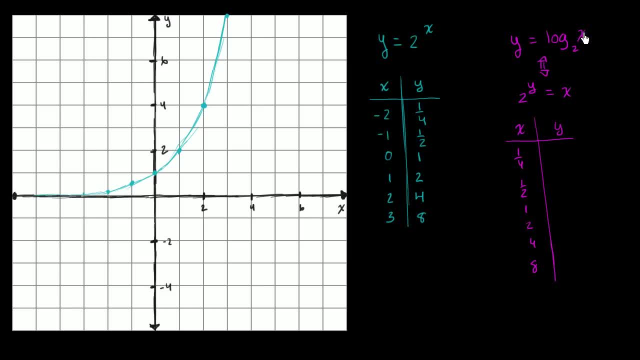 4 and 8.. So here now we're saying: if x is 1 fourth, what power do we have to raise 2 to? to get to 1 fourth, We have to raise it to the negative 2 power. 2 to the negative 1 power is equal to 1 half. 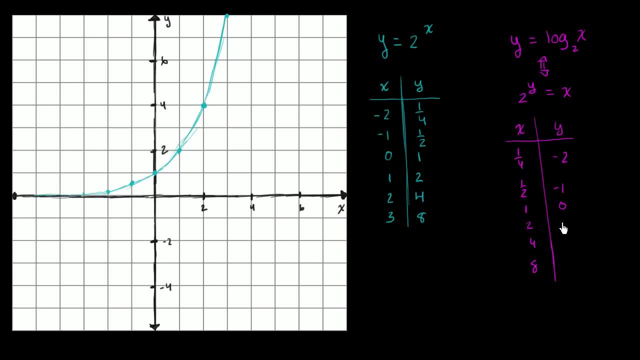 2 to the 0 power is equal to 1.. 2 to the first power is equal to 2.. 2 to the second power is equal to 4.. 2 to the third power is equal to 8.. Notice all we did. is we essentially? 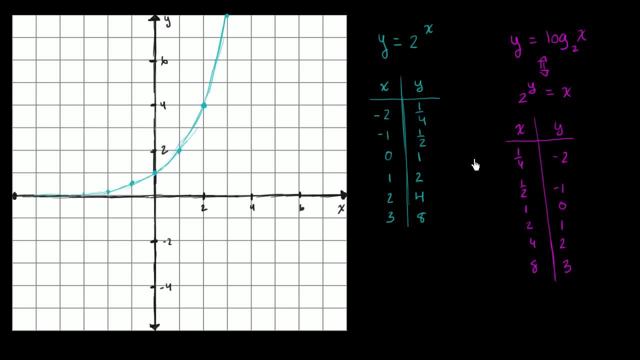 swapped these two columns, And so let's graph this: When x is equal to 1, fourth y is equal to negative 2.. When x is 1, half y is equal to negative 1. y is equal to negative 1.. 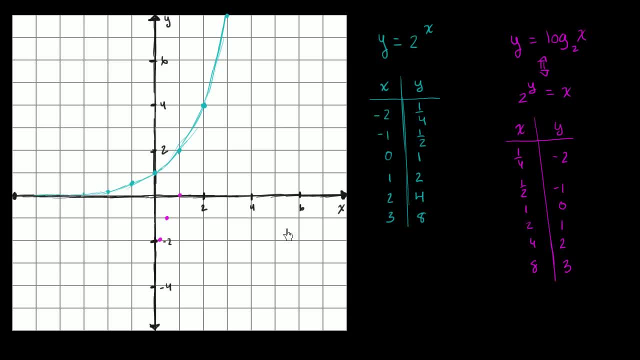 When x is 1, y is 0.. When x is 2, y is 1.. When x is 4, y is 2.. When x is 8, y is 7. 3. So it's going to look like this. 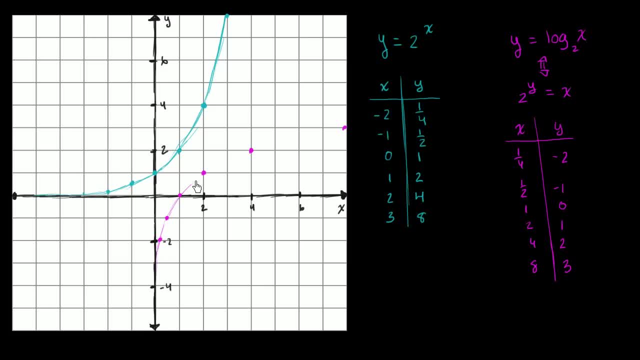 So notice, I think you might already be seeing a pattern right over here. These two graphs are essentially the reflections of each other. And what would you have to reflect about to get these two? Well, you'd have to reflect about: y is equal to x. 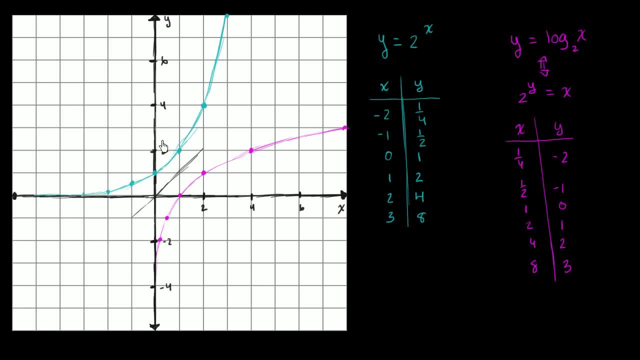 So if you swap the x's and the y's, so there's another way to think about it. If you swap the axis, you would get the other graph, which is essentially what we're doing. Notice, It's symmetric about that line.